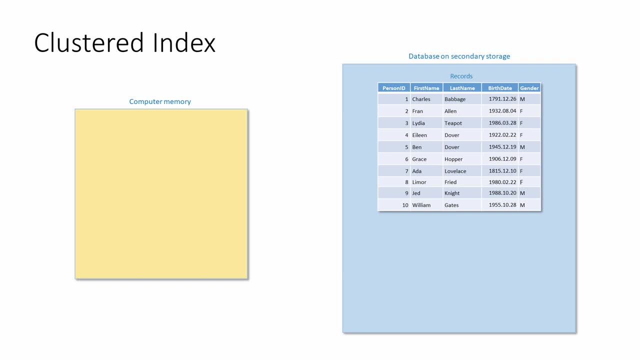 can only have one clustered index, because the records can only be in one particular order. However, a single clustered index can be made up of multiple columns. This is known as a composite index, In the same way that a telephone directory is organised by last name, then first name. If a table has a primary key, this will normally 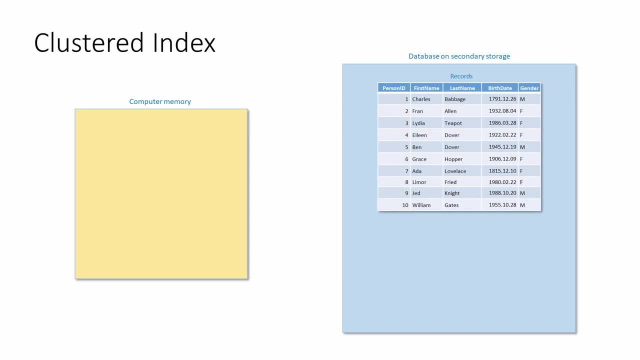 be the clustered index. When a query involving the clustered index is executed, the data on secondary storage can be searched very quickly and the record retrieved to memory. This table doesn't have a primary key and it doesn't have a clustered index. The order: 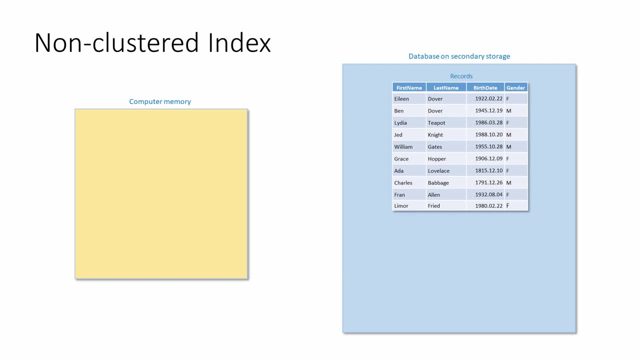 of the records is the same as the table. This table has a primary key and it doesn't have a clustered index. The order of the records is simply the order in which they were added to the table. These records are stored in a so-called heap. This table does, however, have a non-clustered 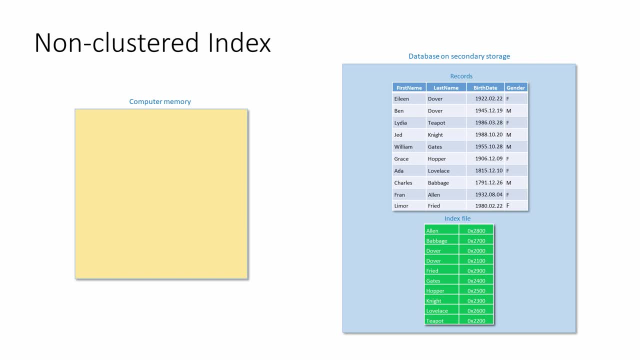 index, also known as a secondary index or a secondary key. A non-clustered index is a separate data structure from the records and it functions rather like the index in the back of a textbook. The data inside a non-clustered index are in order and each. value in the index is a separate value. The data inside a non-clustered index is a separate index and, in turn, a separate index. The number of numbers in the index is a separate value and each value is a separate value. This is due to the fact that the index has 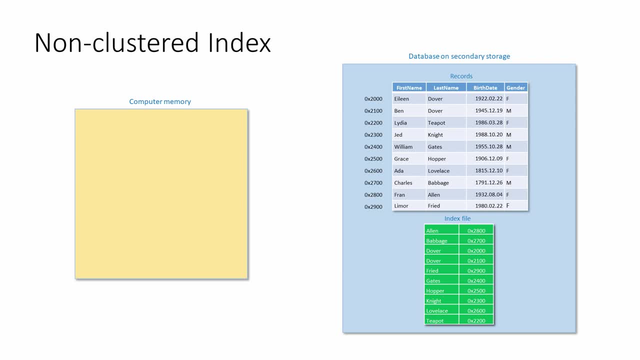 a pointer to the physical location of the entire record on secondary storage. When a query involving the indexed column is executed, a copy of the entire non-clustered index is loaded into memory. This is then searched for any matches. When a match is found, the entire record is retrieved from secondary storage, Because the computer's 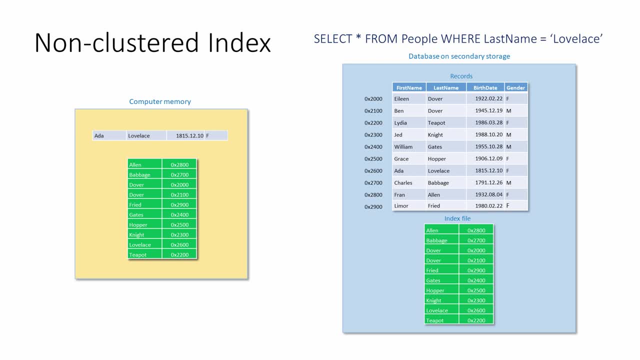 RAM can be accessed much faster than secondary storage. searching the index is very quick, indexes very quick and because the index is ordered, a binary search can be used, which is particularly fast In some database systems. a non-clustered index is a binary tree data structure which 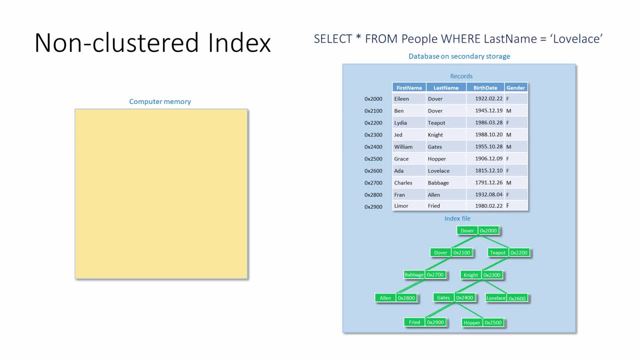 lends itself to fast searching. A table can have several non-clustered indexes, so you can index as many different columns in a table as you like, but whenever you change, add or delete data, each index on disk has to be updated immediately.